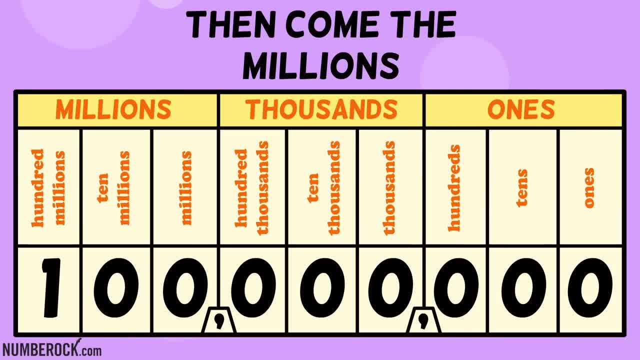 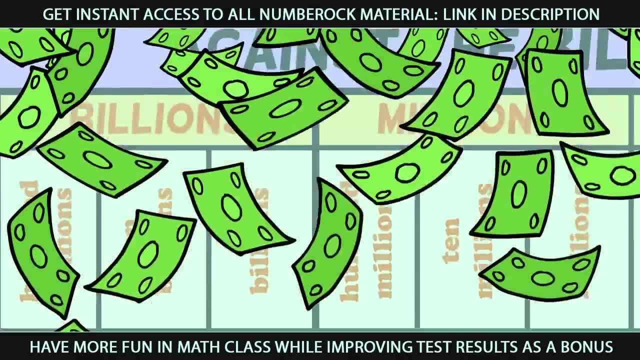 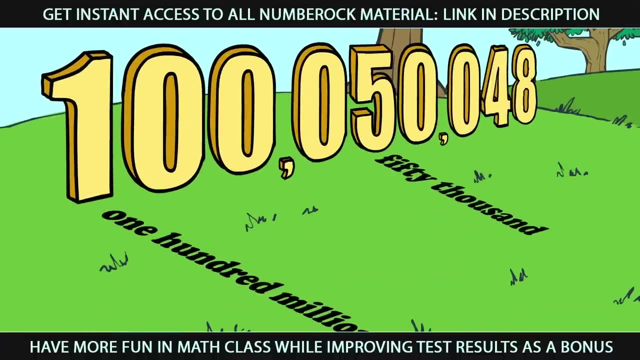 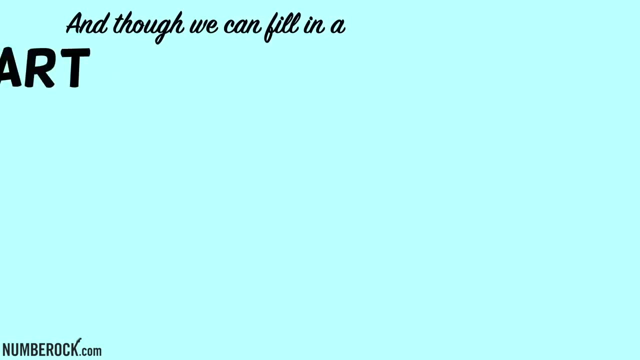 Then come the millions: One millions, ten millions, hundred thousands, And when we get that far we're brushing up against the billions. One hundred million fifty thousand forty-eight. The word form is what we speak to communicate All we can feel in a place value chart. 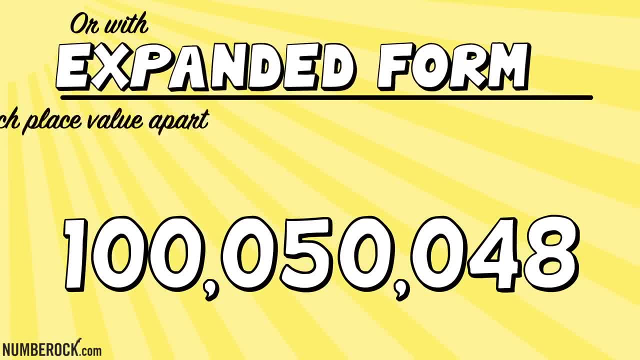 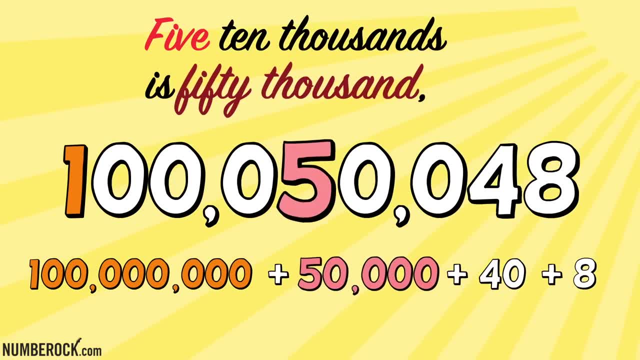 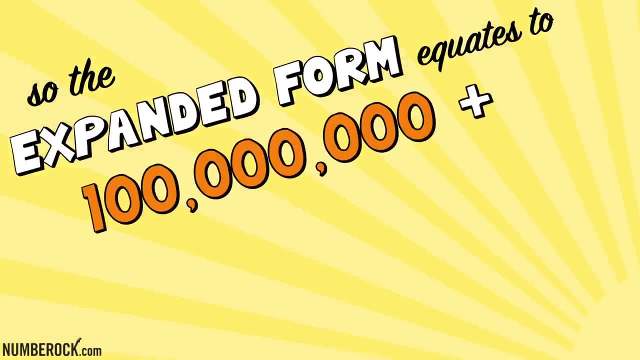 All we'll expand and form break each place. There's just one group of one hundred million. you see, Five ten thousands is fifty thousand, and four tens is forty. Eight ones makes eight. so the expanded form equates To one hundred million plus fifty thousand, plus forty plus eight. 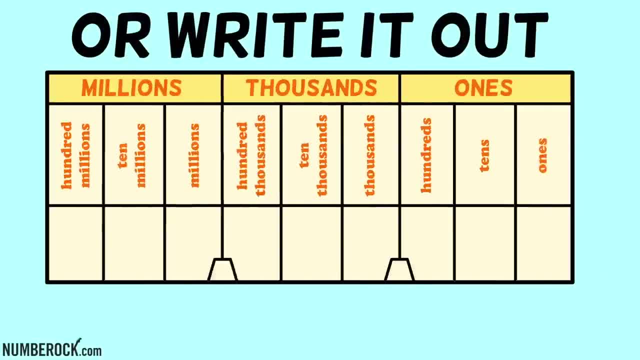 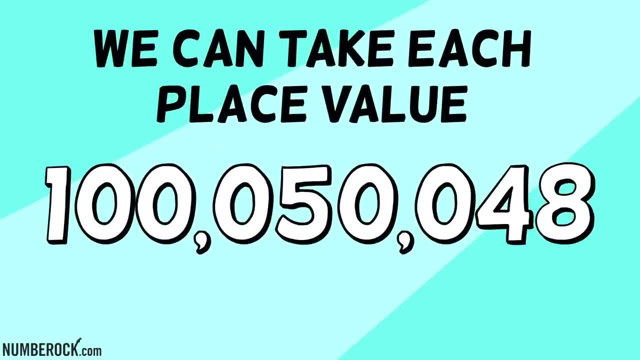 Now check it out. We can say a number, his name or write it out On a chart. We can take each place value and then We can say a number, his name or write it out. We can take each place value and then We can break it apart. 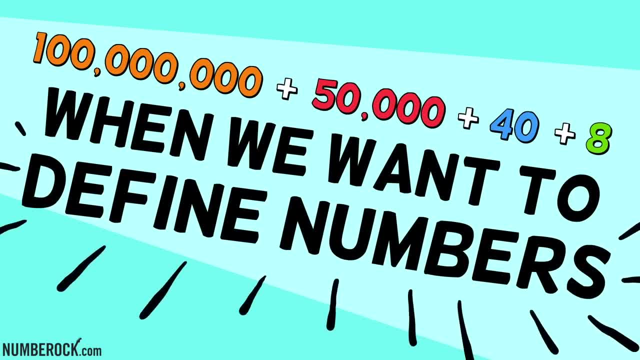 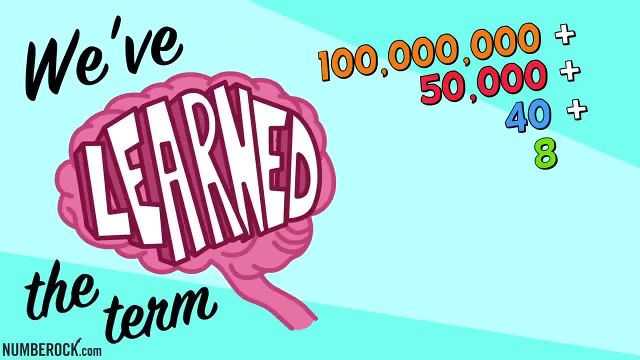 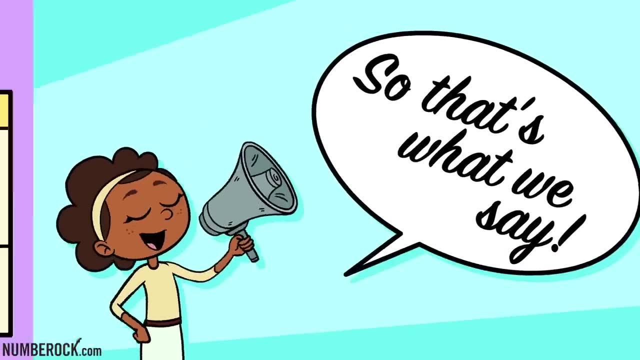 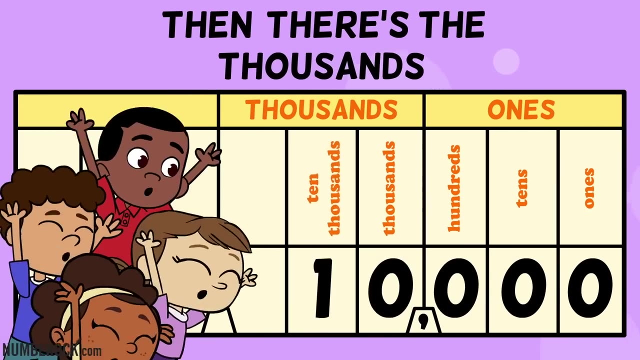 When we want to define numbers written in this way, We've learned the time expanded form. So that's what we say: First there's the ones- Ones, tens, hundreds- Then there's the thousands: One thousands, ten thousands, hundred thousands. Then comes the millions: One thousand, ten thousands, hundred thousands. 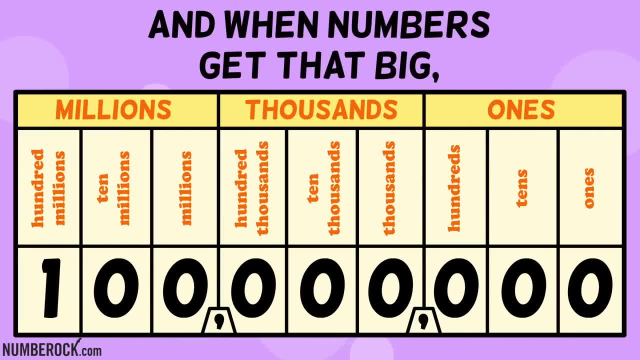 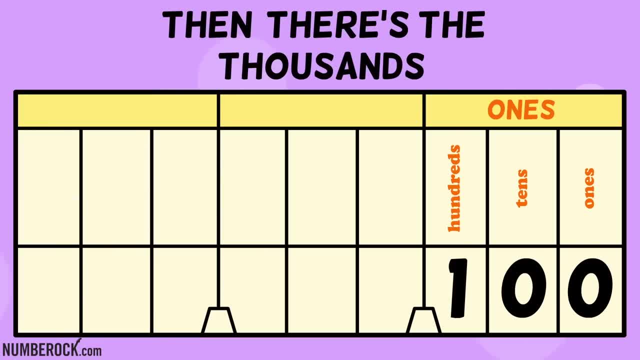 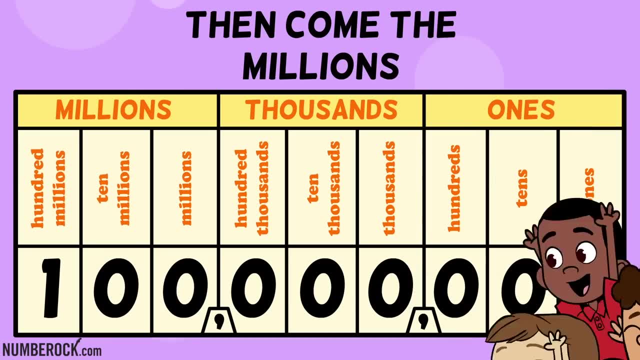 One million, ten millions, hundred millions. And when numbers get that big, we're getting real close to the billions, The ones, Ones, tens, hundreds. Then there's the thousands, Ones, thousands, ten thousands, hundred thousands. Then comes the millions: One million, ten millions, hundred millions. 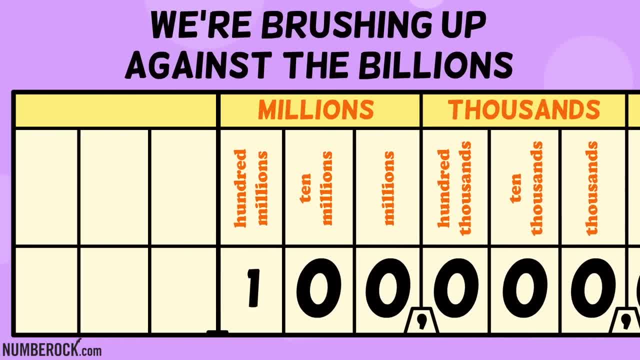 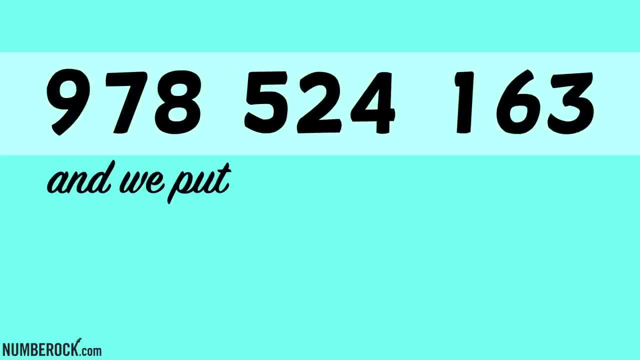 And when we get that far we're brushing up against the billions. The digits and big numbers are in groups of three places. Groups of three are called periods And we put commas in the series Spaces from right to left. We can label them ones, thousands, millions. 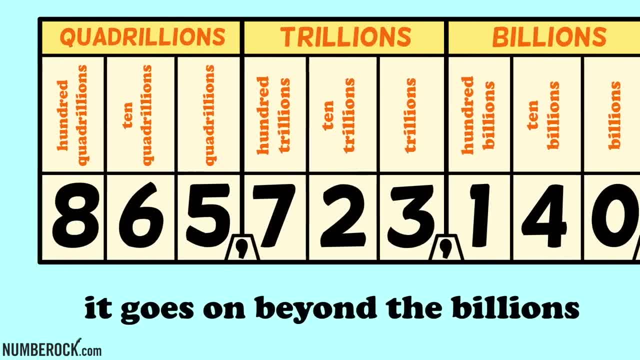 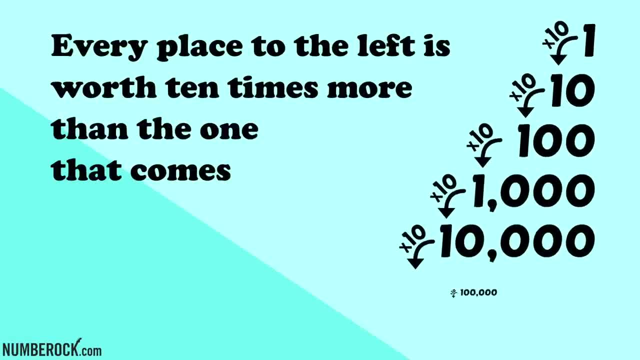 And a large enough number. It goes on beyond the billions. And now's the time for one final line About the base ten number systems design. Every place to the left is worth ten times more Than the one that comes before, And each period we move left Is one thousand times greater.